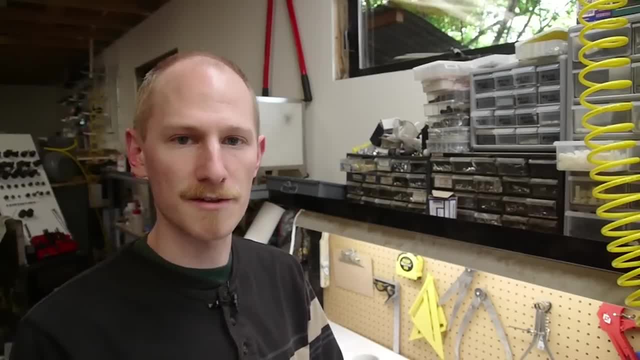 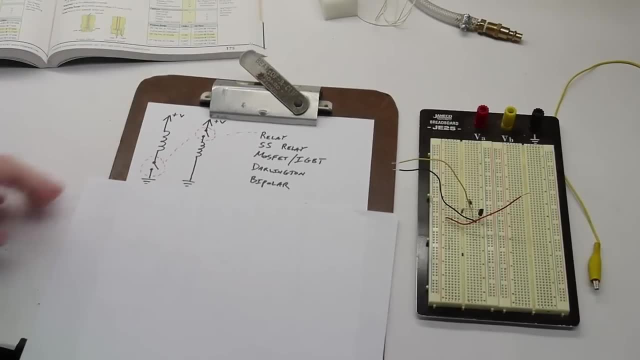 motor or solenoid or something. So this video will show you how to size the transistor and set it up. So let's zoom in and I'll show you what I've got. Okay, so one of the most common tasks that I need to do with a transistor is just to turn something on or off. 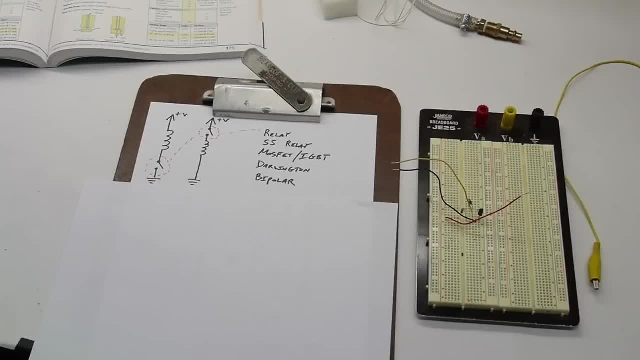 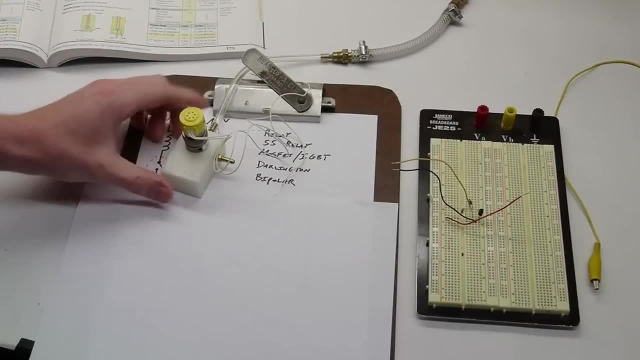 So not really amplifying a signal, It's just acting as a switch. So I drew a couple of diagrams here Today we're going to be controlling this, which is an air valve, a solenoid air valve, and it's a 12-volt device. 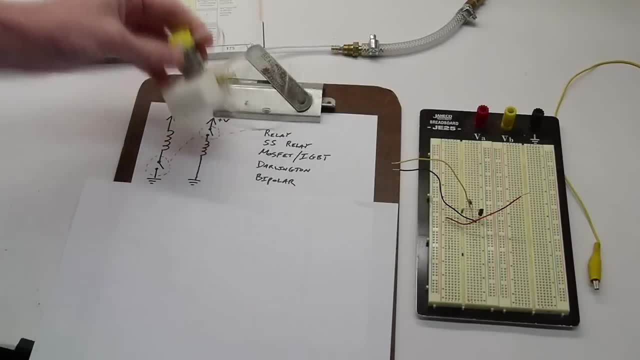 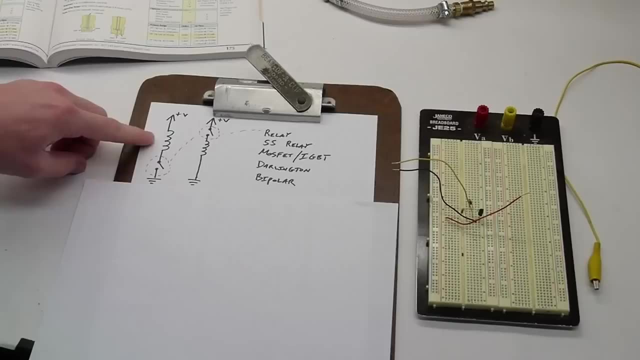 I just put power on it and it opens- Pretty simple. So I just drew it in this diagram. It's a coil, which is a good way to represent it. It's like an iron core coil. So to turn the thing on and off, we could either put a switch between the coil and ground or 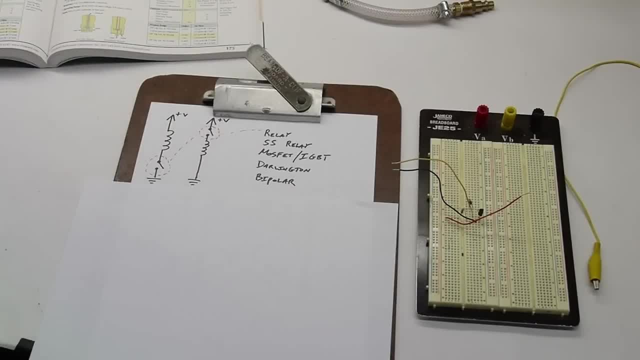 between the coil and our voltage source. It doesn't really make any difference to the coil, but it will make a difference to us later if we choose a switching component. So I listed off a few of them and I'll describe why I didn't pick, why I did or didn't pick them for this project. 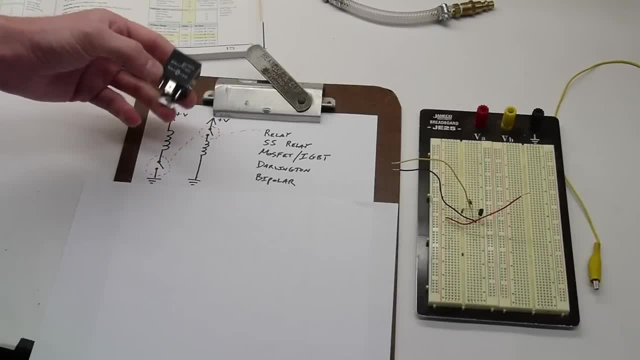 We could have used a relay. It's a bit overkill. In fact, this one is quite overkill. It's big and expensive. It's mechanical. It doesn't switch very fast. The best things about relays are that they can handle very high currents and they isolate the circuit. 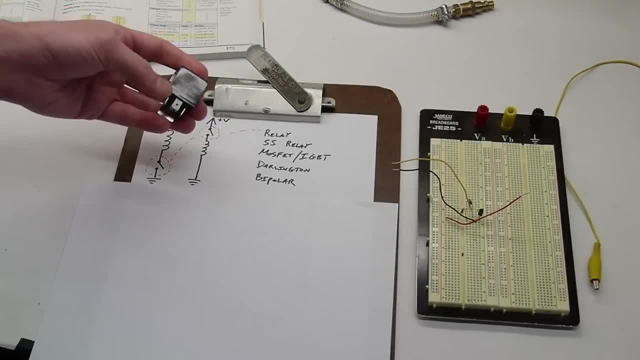 They isolate what is being switched from the control circuit, So we'll save that for another day. Similarly, a solid-state relay, Also a very cool component, Mostly used for isolation and high voltages or high currents. So save that one. A MOSFET or an IGB. 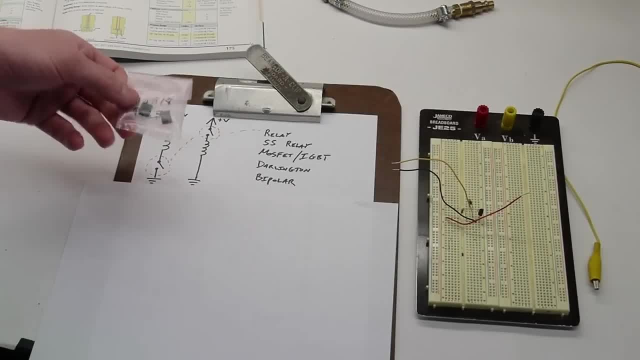 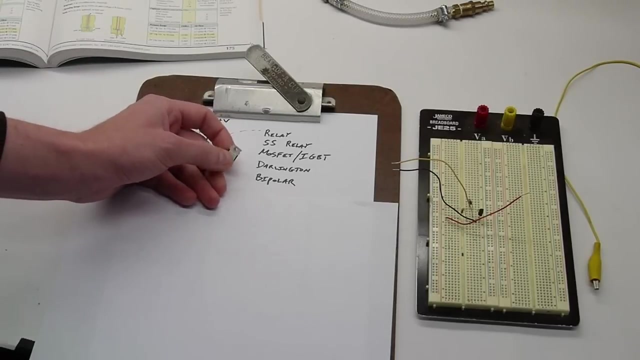 Also for much, much higher currents. They don't isolate. Well, I guess they sort of could, but we're not going to use these today either. A Darlington transistor: This is actually not a bad choice Today. we don't need to use a Darlington. 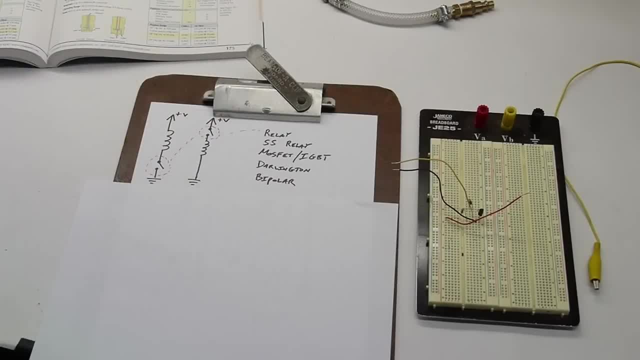 but I think I'll probably do a video on these later because they actually are quite useful on some circuits, Generally for higher current stuff. Today, that solenoid doesn't really use that much current, So we're going to use this little guy. 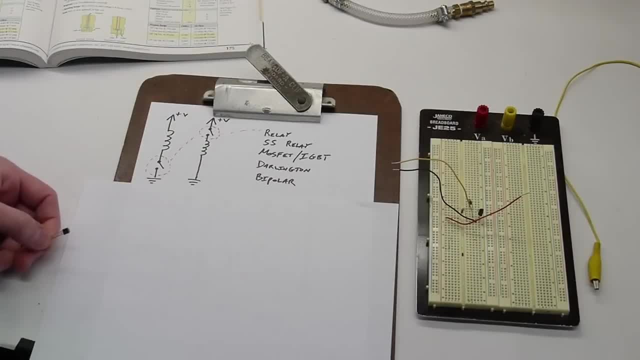 A standard bipolar transistor. Bipolar is just a plain transistor. That's what bipolar means, And this one happens to be a PN2222A, and this little tiny case here is called a TO92 case. So the next thing, the first thing to do when picking a bipolar transistor, is to decide whether we're going to use NPN or PNP. 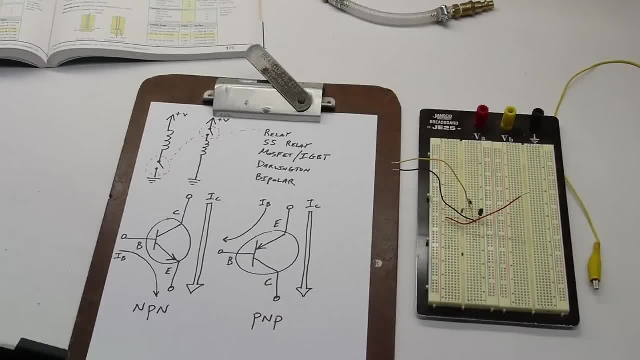 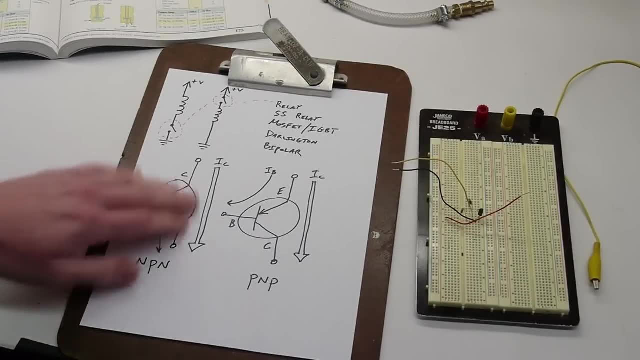 You may have heard these terms before. They're just floating around, So I made a little diagram here to help us decide which one we're going to use. First off, the schematic symbols: The arrow in the symbol always is in the direction of the conventional current flow. 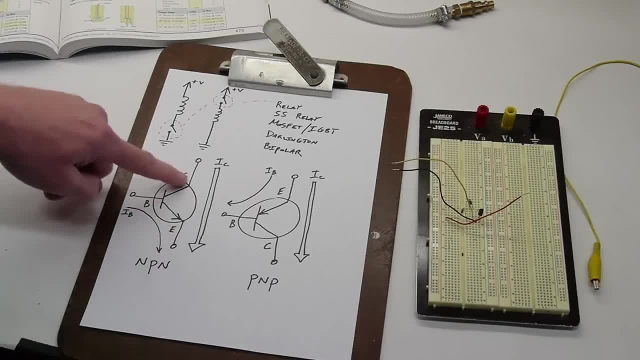 And the arrow always points to the N material, so NPN or PNP. So that's one way to remember it. Also, watch out: I switched the emitter and collector between these two in the diagram here, So it's collector base emitter, emitter base collector. 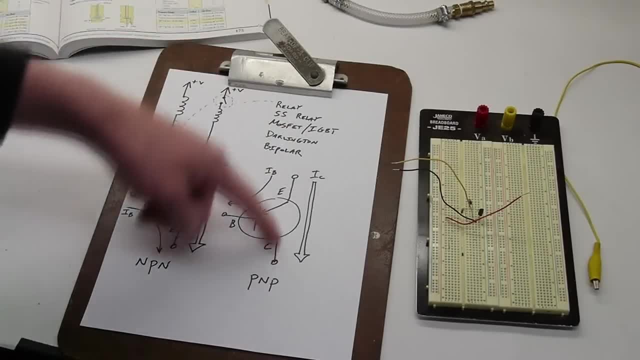 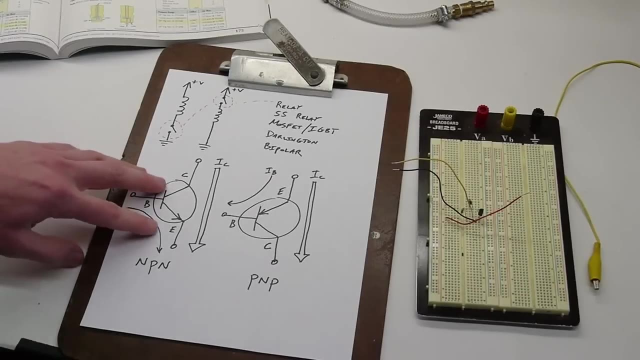 So in a PNP, the conventional current flow goes from the emitter to collector, and in an NPN it goes from collector to emitter. So you may be wondering, well, you know, what can we do with all this? Basically, what we're going to do is put one of these in place of 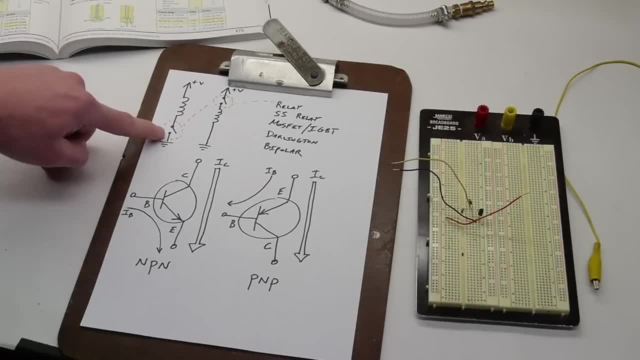 the switch here, And the two terminals of the switch are going to be the collector and emitter or emitter and collector, depending where we put it in the circuit here. And the way that we get these switches to turn on or off is by either pouring current into the base. 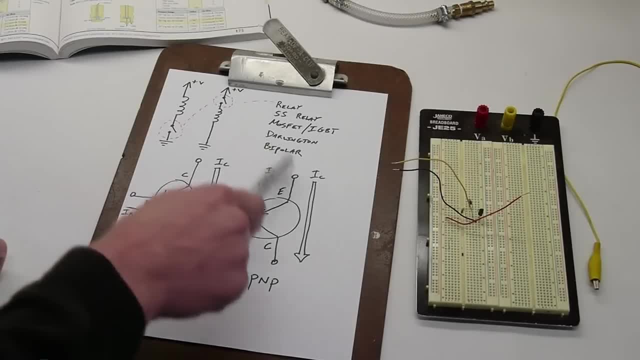 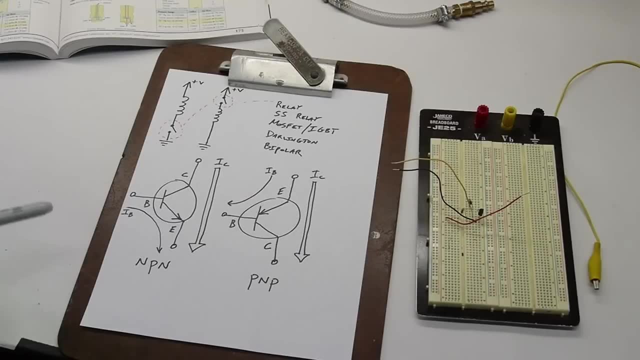 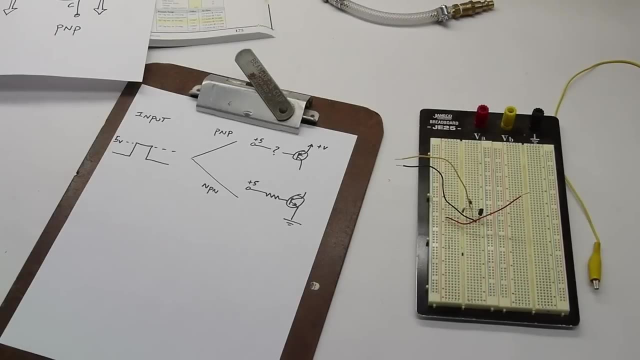 in the case of an NPN, or drawing current out of the base, in the case of a PNP. So it's a switch that is controlled by a current flow. Okay, so a minute ago I said that a transistor is a switch that is controlled by a current. 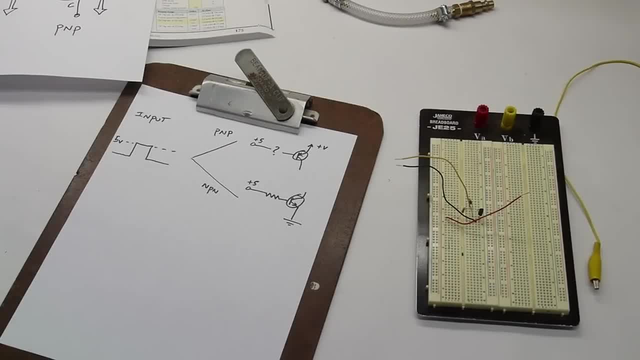 flow and that we were trying to decide between PNP and NPN for our circuit. So how do we actually decide? In this case, the thing that's going to make the decision for us is our control signal, And in this case it's going to be our favorite zero to five volt logic signal that this could. 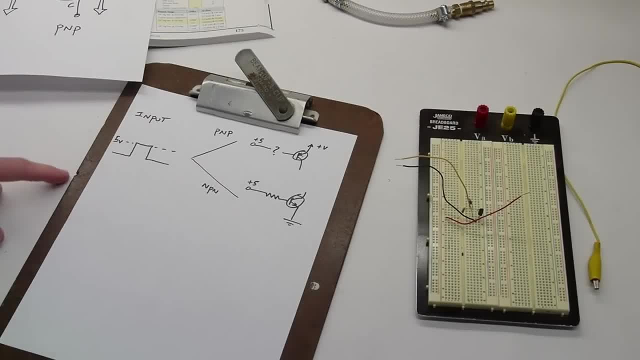 come from a microcontroller or a PC parallel port. There are a number of different things, So let's look at each case. If we went for a PNP transistor and we have this- either zero volt or five volt control signal- we don't have an easy way of controlling how much current is going to flow out of the 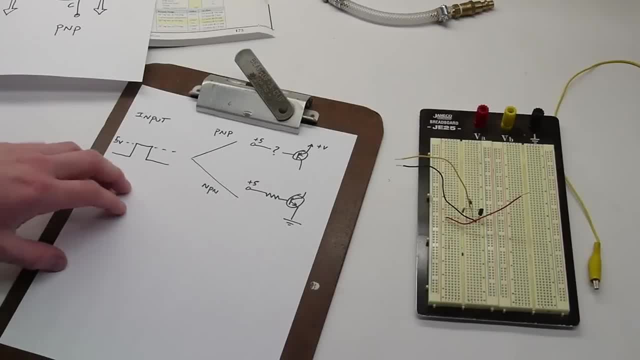 base of the transistor to turn it on and off. And the reason for that is, if the base is at five volts or we have a five volt signal and then there's some sort of circuitry between it and the transistor, there's going to be 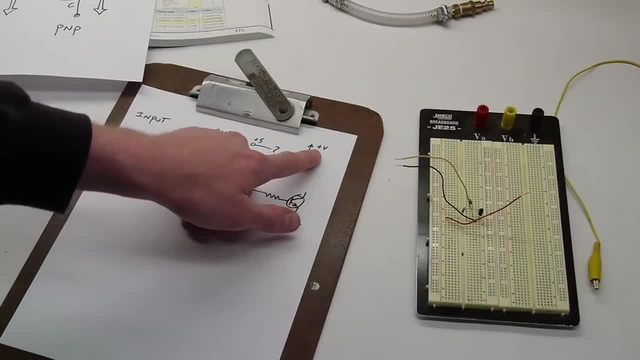 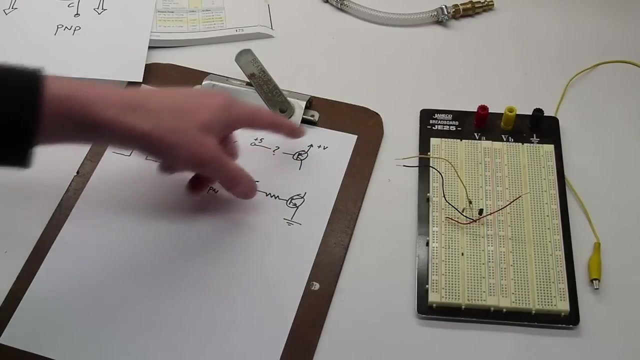 a current flowing from our PNP Supply voltage. in this case it's like 12, but it could be a number of different things And in the two cases of the base being zero or five, there isn't really an easy piece of circuitry we can put here that will allow us to control the base current flowing from. 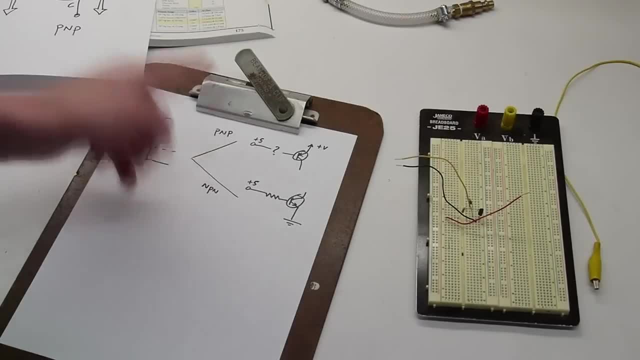 the emitter to the base in the case of a PNP. However, in an NPN transistor we have a really great option. It's just a resistor. So when this is at five volts, We have a current flowing from the base to the emitter and that's going to turn the 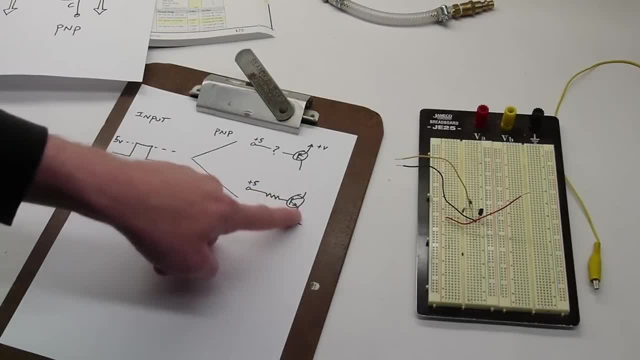 transistor on And when this is zero, no current is going to flow and the transistor will be off. So this is perfect. So in this case, the NPN is an obvious choice. In fact, in all of my projects, I probably use NPN transistors 95% of the time. 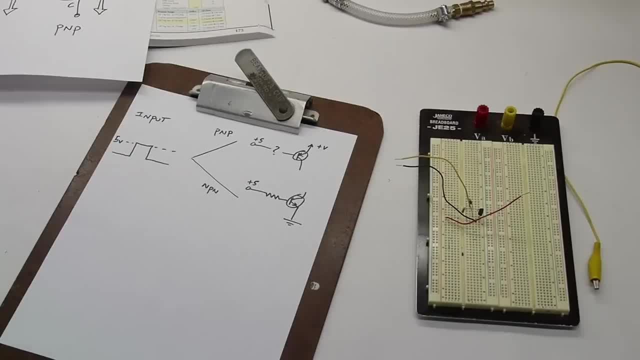 In switching applications like this, I think you would almost always want to use an NPN, So just keep that in mind. I think, in general, NPNs are quite a bit more common, So let's talk about actually choosing a transistor and setting it up with this solenoid valve. 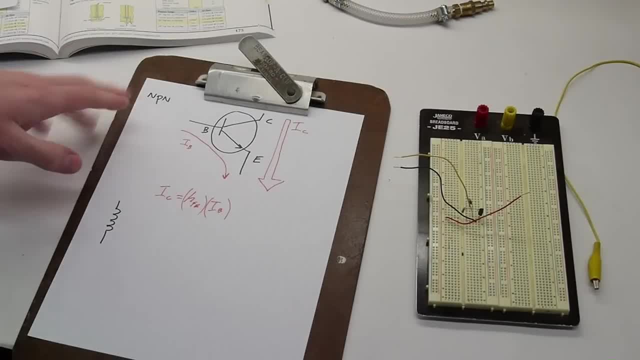 So we've decided to go the NPN route because it's easier for us to control the base currents with an NPN in the type of circuit that we're using here, And I said that a transistor is a current amplifier or a current controlled switch. 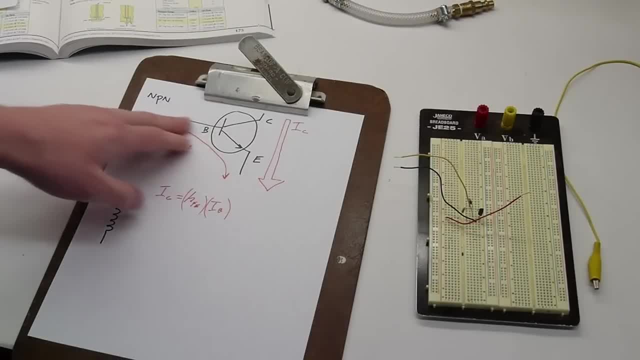 So if we pour some current into the base and it flows From the base to the emitter, that will turn the transistor on and allow a large current to flow from the collector to the emitter, And the amount of amplification is known as the transistor's gain. 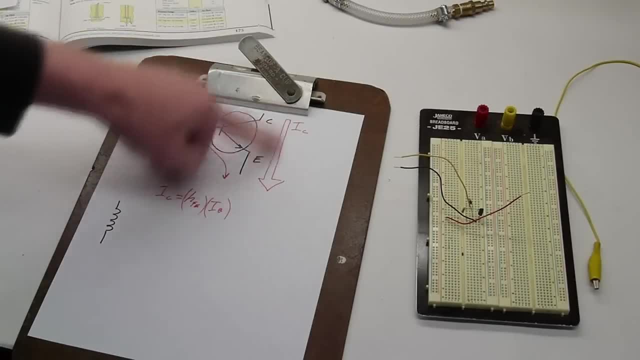 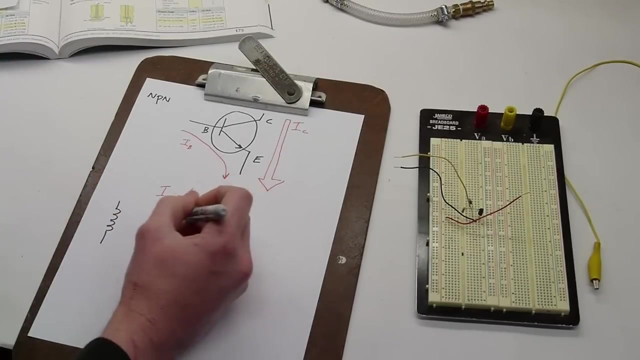 So a transistor with a high amount of gain will allow a large collector current to flow with just a small base current, And a transistor with not much gain will not have as much amplification. And that amplification factor is known as HFE, Or it's also sometimes called beta. 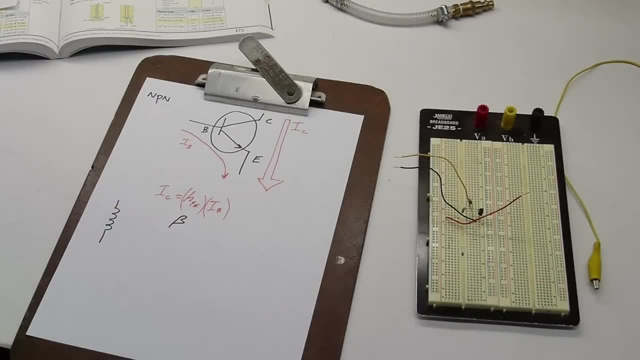 That's the gain of the transistor at DC. I should also point out that we're not talking about AC circuitry here at all. This is all just steady state DC analysis to make our lives easy. So what we're going to do here is pick a transistor. 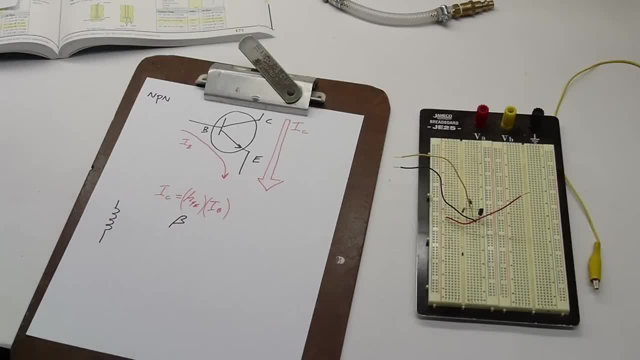 And this is a little bit where, you know, experience comes into play. I mean, there's thousands of transistors available. How do you pick one? Well, you know, for hobby projects and sort of small stuff, For small scale design like this, there's really only a handful that come up. 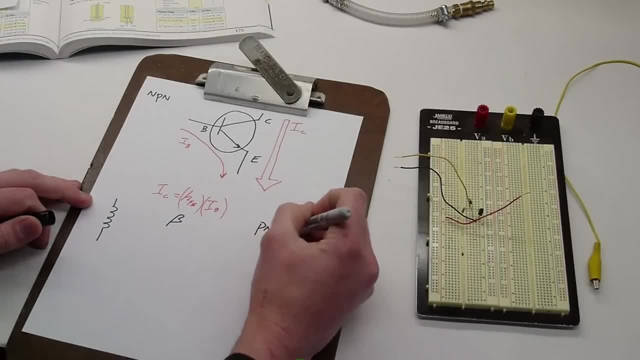 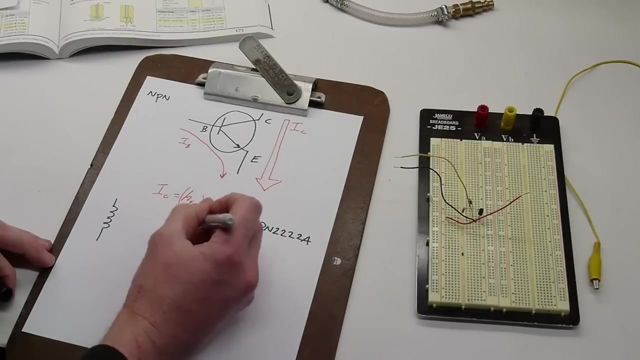 So I'm just going to say that we're going to pick the PN2222A, which is a really great low medium power, very inexpensive, easy to use switching transistor And it has a beta of about 100.. We could be more conservative than that, but we'll just say beta is 100 for this particular. 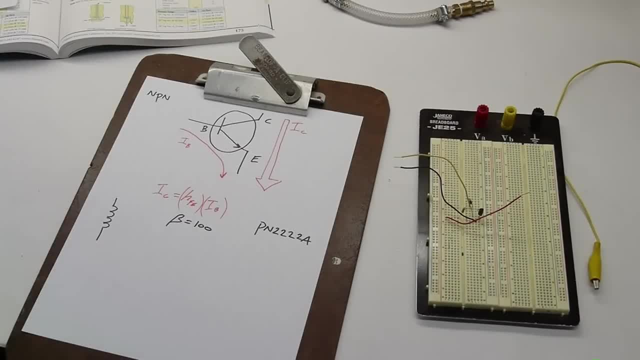 transistor. So it varies quite a lot. And I mentioned Darlington transistors earlier. Darlington transistors are basically two transistors ganged together to increase the gain. So those can have gains of, like you know, 10,000 or something. 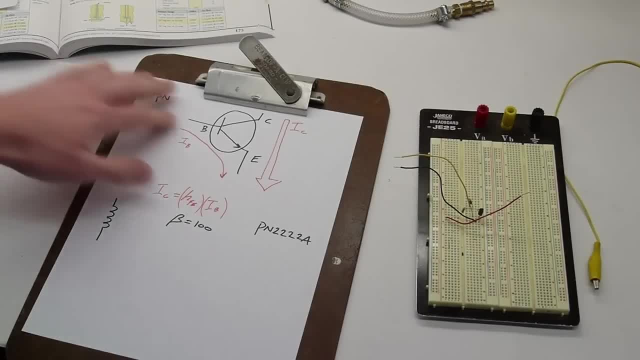 And that could be quite useful for switching higher current loads while keeping your base current low. So, anyway, so let's get back to the design that we're actually doing today. this solenoid valve, This is a clippered solenoid valve. 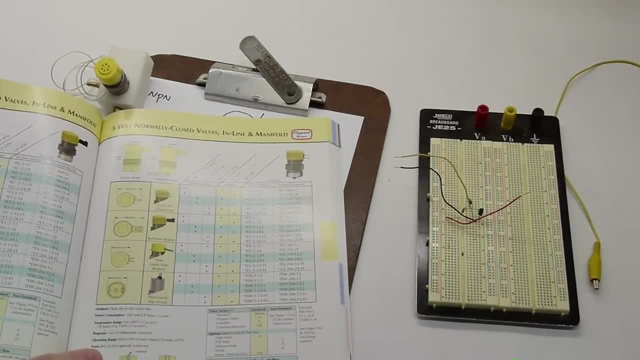 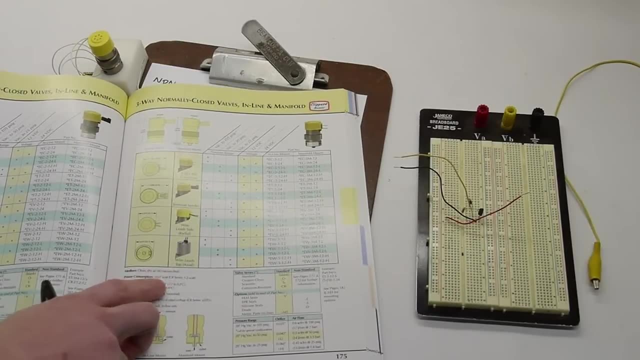 And if we get the spectrum, If we get the direct sheet in here, there's not very much for electrical specifications. It just says 0.67 watts at 12 volts. They make this in 12 or 24 volts. This is a 12 volt variant. 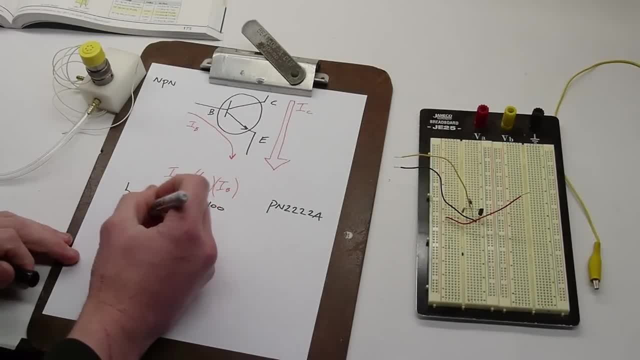 So we've got our schematic representation here: 0.67 watts at 12 volts. Well, we want to know the current, So we use Ohm's law, which is current times voltage. Current times voltage equals power, or in this case we want to go in reverse: 0.67 watts. 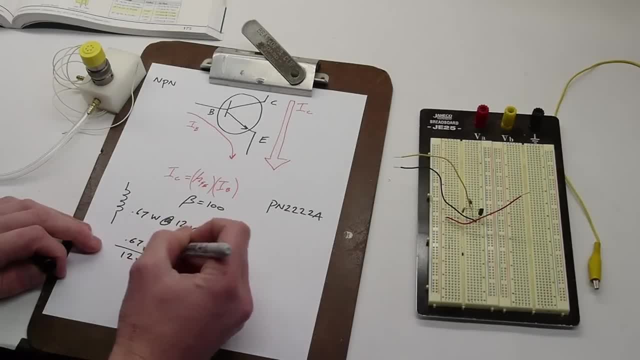 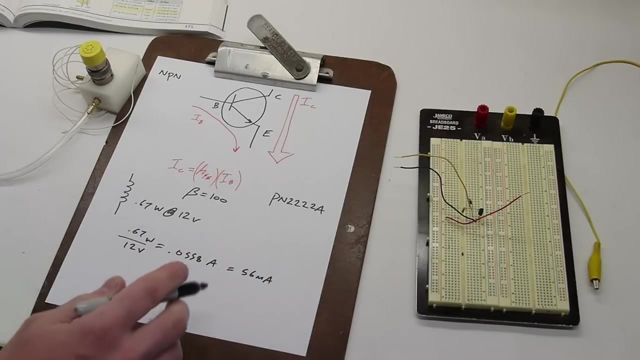 over 12 volts. Put some units on there for you. I just type this one up- is 0.0558 amps or about 56 milliamps. Okay, So if we didn't know which transistor we were going to use, You could just start looking down the list of transistors in a catalog and think to yourself. 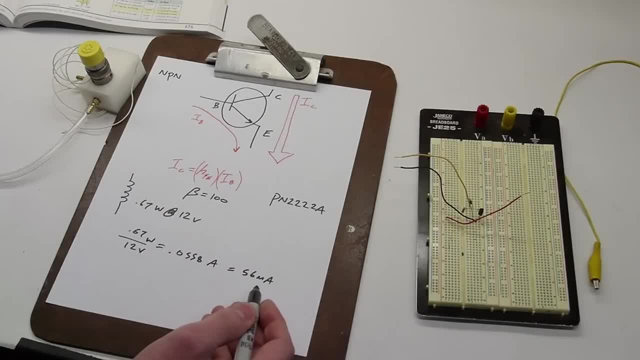 well, the transistor is at least going to have to handle 56 milliamps, Although you'll find that pretty much every single transistor can handle more than this. This is not a very big requirement here. So what we know at this point is that we're going to use an NPN transistor. 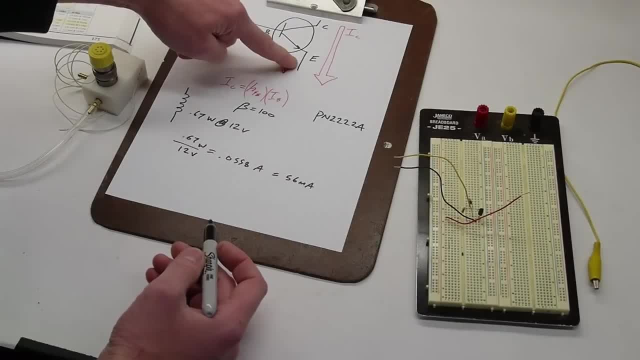 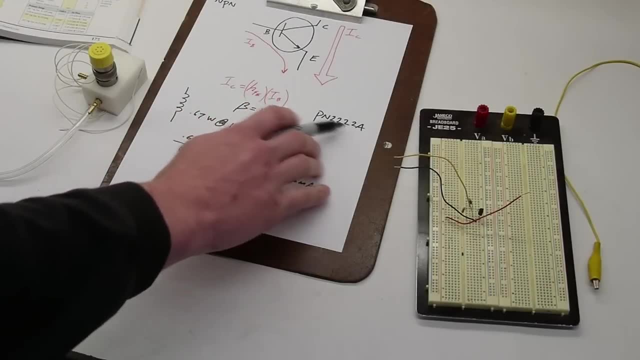 It has to handle 56 milliamps from the collector to the emitter. And now we need some way of turning the thing on and off. And if we did decide to use the PN2222A, we know that its beta is 100.. 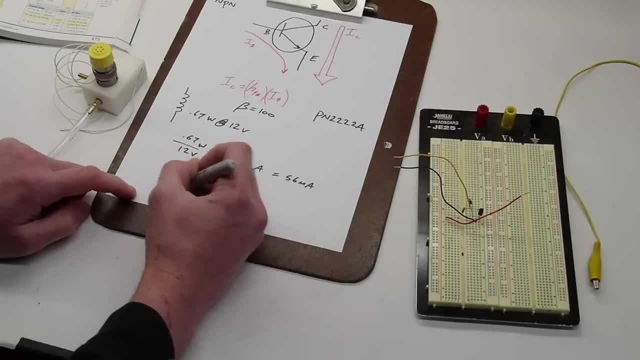 So what we have here is our transistor And IB. the base current is flowing like this: This is grounded, This is the coil with our voltage source And this is This is the collector- current flowing through the coil to ground. And I said that beta is 100, meaning that this is 100 times less than the collector. 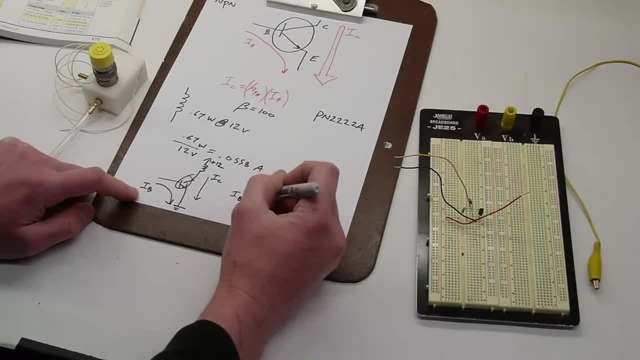 current. So IB is equal to 56 milliamps over 100, or 0.56 milliamps. So now the question is: how do we get 0.56 milliamps to flow into the base? Luckily, there's a really easy way. 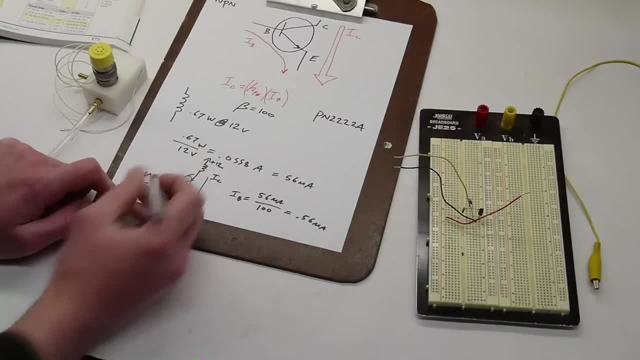 We can just add a resistor. So if we put a resistor here and then send this over to plus 5 volts, if we size the resistor correctly, we'll get exactly 0.56 milliamps to flow through here. The transistor will multiply it by 100, and we'll get the current to flow through the. 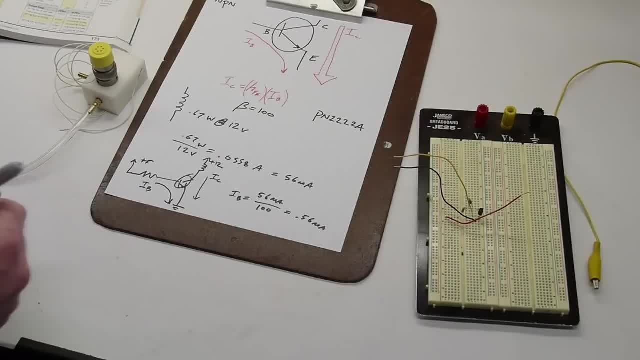 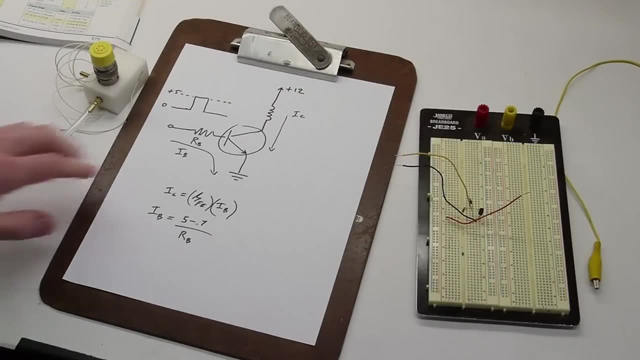 coil. So let me draw this a little bit more clearly and then we can choose our resistor value. So our circuit is almost done. This is a pretty good, almost finished version of it. here We've got a resistor on the base where we're going to put our 0 to 5 volt signal and the 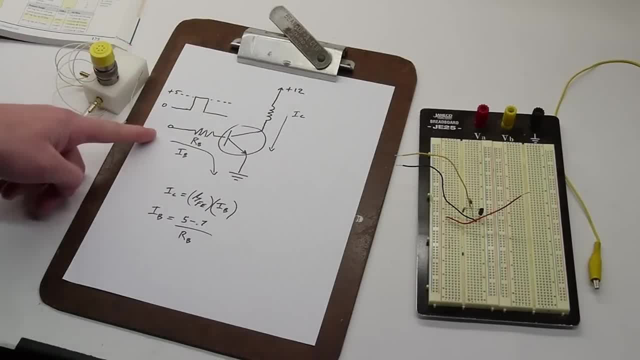 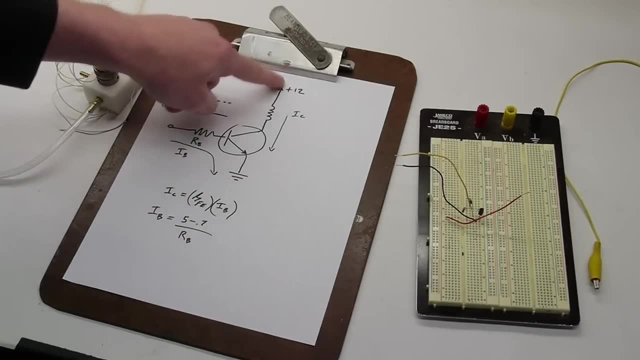 coil is connected here, The solenoid is connected here, So that when the input is 5 volts, we get a current flowing through this resistor which turns the transistor on and allows a large current to flow through the coil to ground. So you're thinking, yeah, but I live in a voltage world. 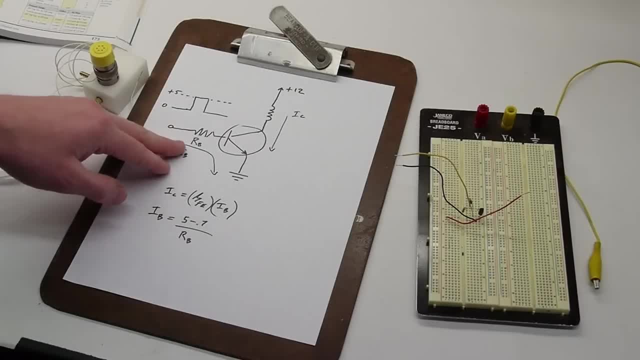 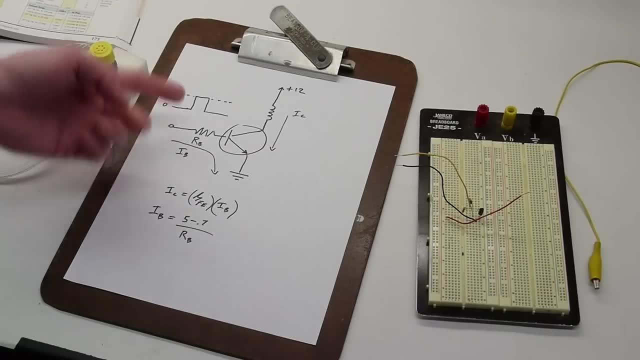 How do we actually get this thing to turn on and off? So we put this resistor here to convert our input voltage to a current. and you might be thinking: well, that's easy. I'll just use Ohm's law. Five volts over the resistor value gives me the current. 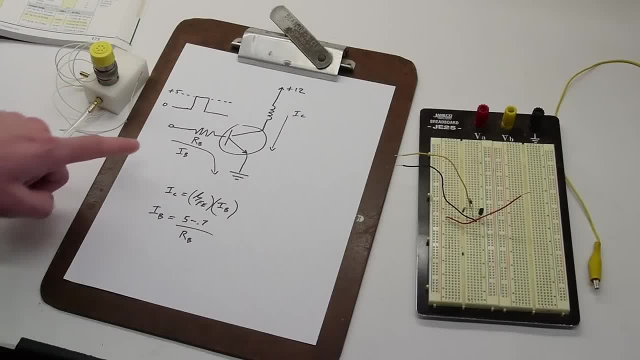 Almost. There's another little twist here. The base current is actually 5 minus 0.7 divided by the base resistor, and this 0.7 is an intrinsic value to silicon transistors. This is an NPN, So there's a PN. 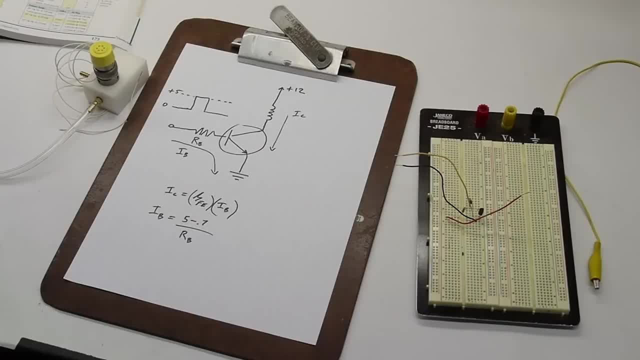 Junction here And silicon PN junctions will drop a voltage, And for pretty much all transistors I think it's about 0.7 volts. I think it's 0.6 volts for diodes. I'm not exactly sure why that is, but you can look that up. 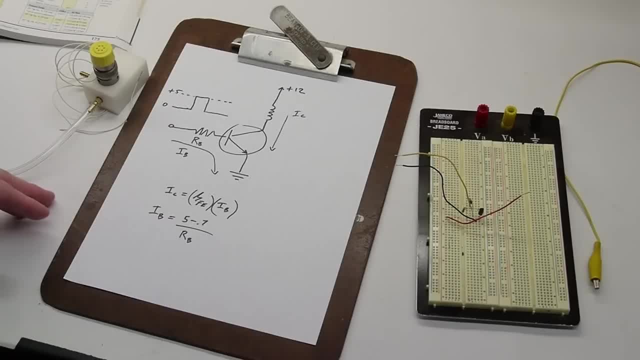 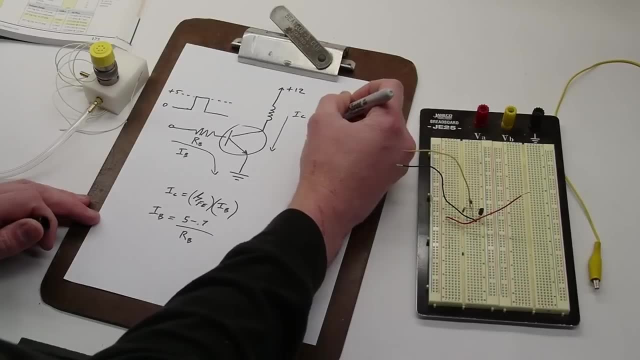 And so we know that to get our coil working, we needed 56 milliamps to flow. So the IC has to be, let's say, equal to 56 milliamps. So that's that. So that's that. That's that. 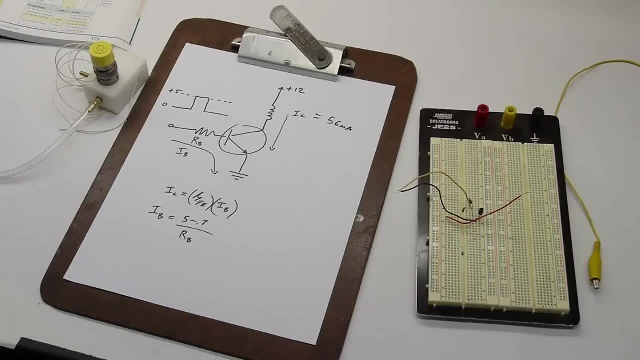 And I said that the transistor amplifies current by 100. So we need at least 0.56 milliamps to flow through the base. But it's actually a better design practice to shoot a little bit higher because we want to make sure that the transistor is fully on. 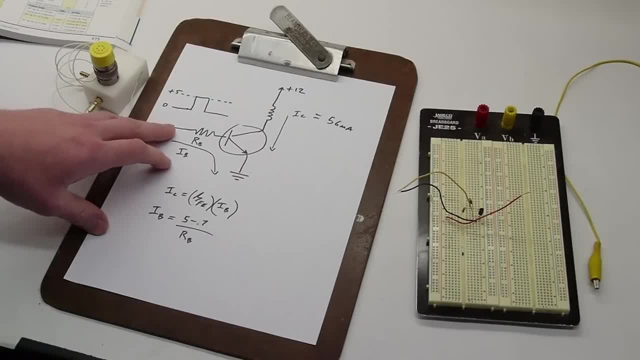 What would happen if we gave it less base current. Let's say we only gave it 0.1 milliamps in the base. So you'd multiply that by 100. And we get 10 milliamps flowing through the base. 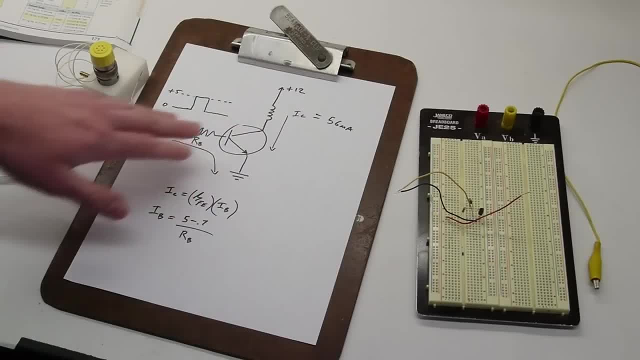 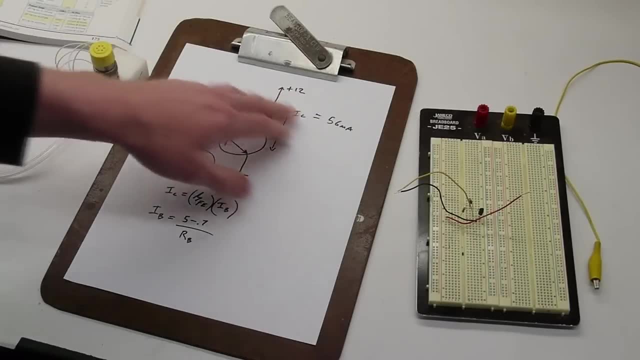 So that's that, And that would not be enough to activate our solenoid. So, the way we have it designed now, if we chose a base resistor that only allowed 56 milliamps to flow through the collector, the circuit would just be on the cusp of working. 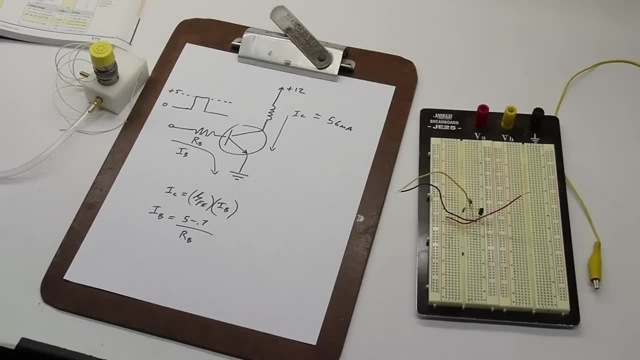 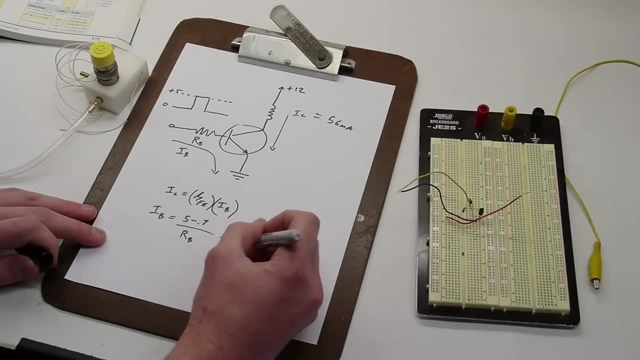 We want to design it to be a little bit safer. So let's just say we want to shoot for a base current of 1 milliamp, So we use the multiplication factor And we get 100 milliamps through here. So you might be thinking: well, wait a minute. 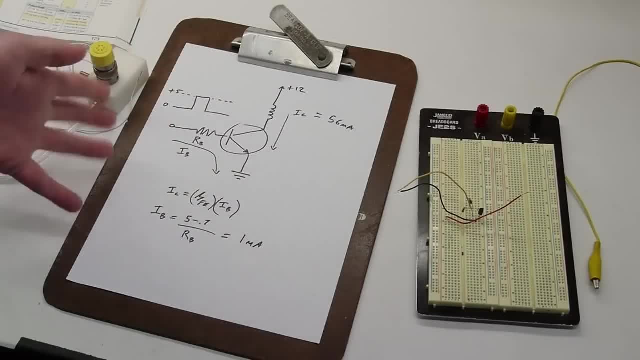 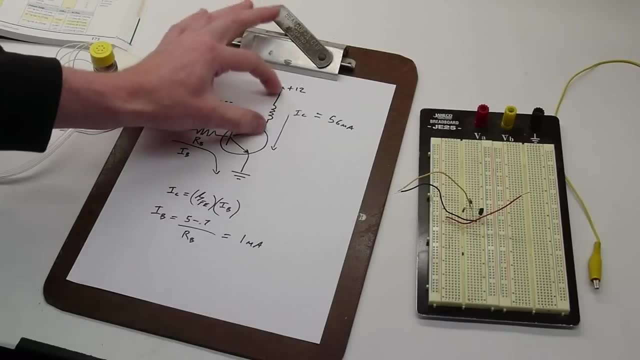 How do we get 100 milliamps flowing through this? The answer is that we actually don't get a full 100 milliamps because the current is limited by the solenoid itself. If we were to connect the solenoid directly to 12 volts and ground, it's only going to. 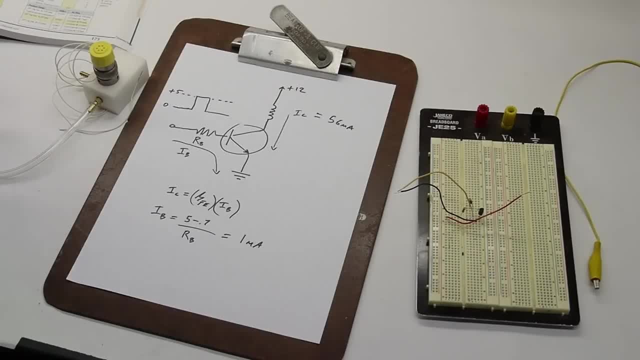 flow as much current as the manufacturer has rated 56 milliamps. So it transits, So it transits. So the resistor can't allow more current to flow through the device than it would normally use on its own, But it can restrict the current. 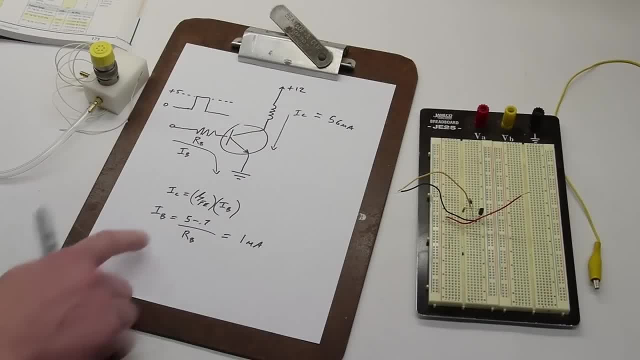 OK, So let's solve this guy. We've got: IB is equal to 5 minus 0.7 over RB, And we know that IB is 1 milliamp. So when doing the calculations, always use the standard units. So enter this as 0.001.. 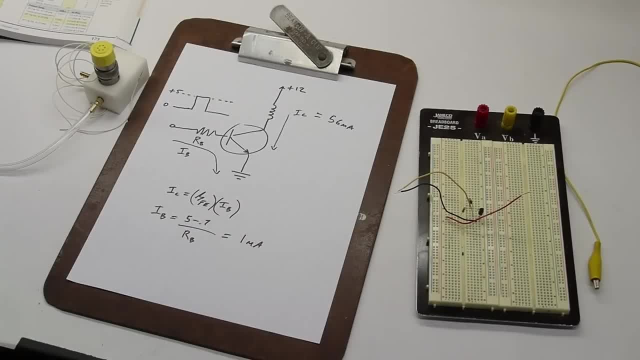 OK, Let's do parish. We have again crazy light resistance. It shows up at 4.9 ami-amp. 0.051.. That's still not the correct number, OK, OK, So 0.07, that's about 3 minutes, so we hit it. 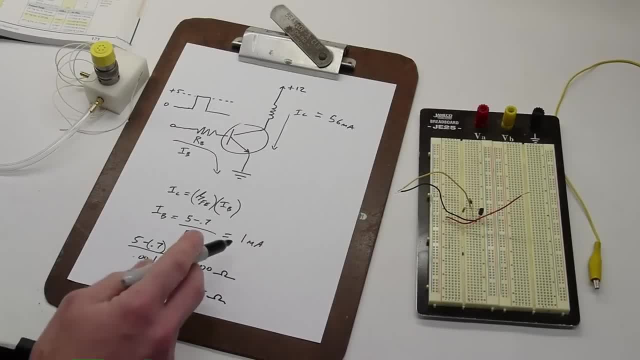 You can see that if you jump to the turns, Portuguese cùng вы pronounce that right. we can see that 0.001 was less than 2 minutes. That's fretting through here. This looks like it would be a shorter current from re- regeneration. 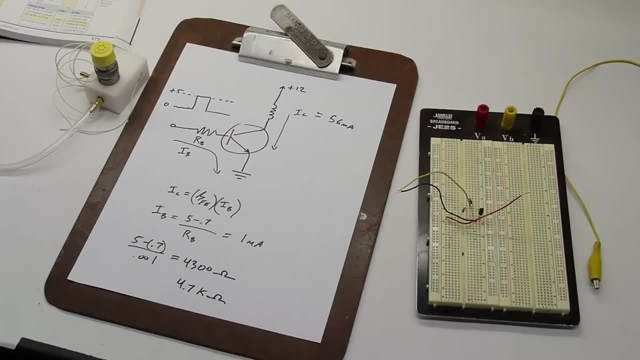 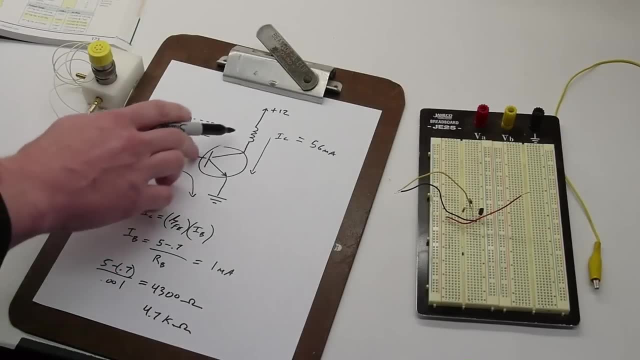 It would be shorter than BB And into the反射 .18 right here. All right, much okay. So there's one other thing I wanted to add here For this particular circuit, since we're switching a coil. it's actually very important that. 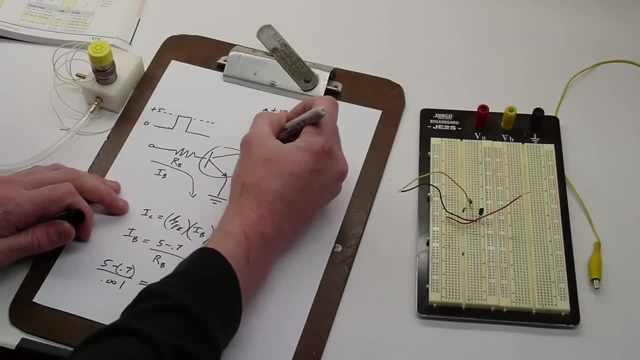 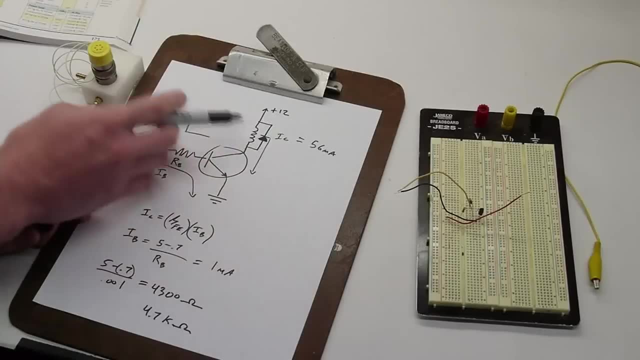 we add a clamp diode and that's going to look like this. So you might be thinking: well, that's stupid. but I mean the diode is pointing into our voltage source. How could this ever get higher than plus 12?? 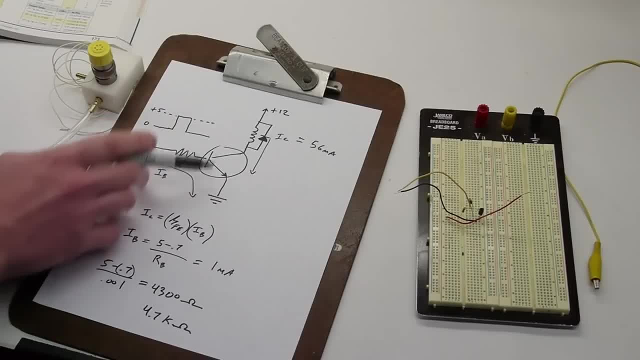 And the answer is that when the transistor turns off, all of that current that was flowing through this coil has created a magnetic field in here, And when the transistor turns off, that magnetic field collapses and the voltage is going to rise at this point. 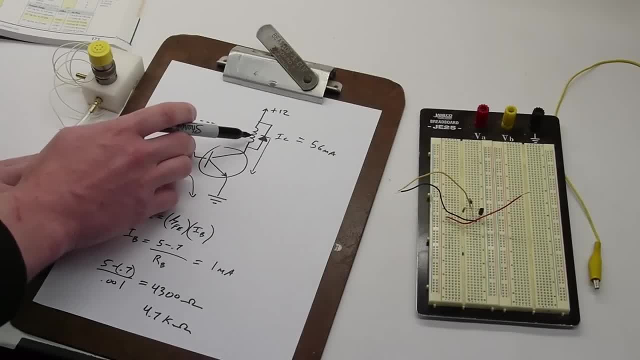 It could be quite significant if the coil has a lot of inductance. the voltage could get to be hundreds of volts here, high enough where it would actually blow out the transistor. So it's extremely good design practice To put a clamp diode in there. it could be a real problem because you might design this and 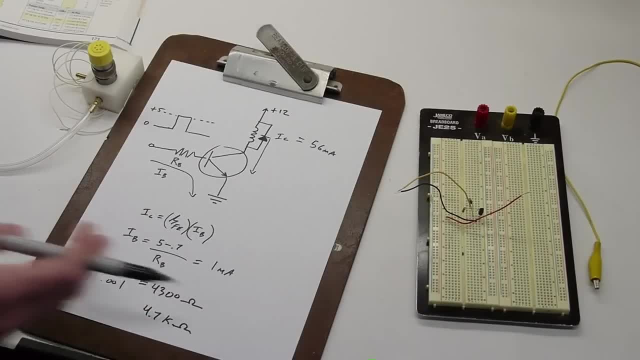 switch it 20 times on the test bench and it works fine. and then you go out and put the circuit into service and it switches and it gets to be just high enough and it blows your transistor out. So definitely put a diode there. 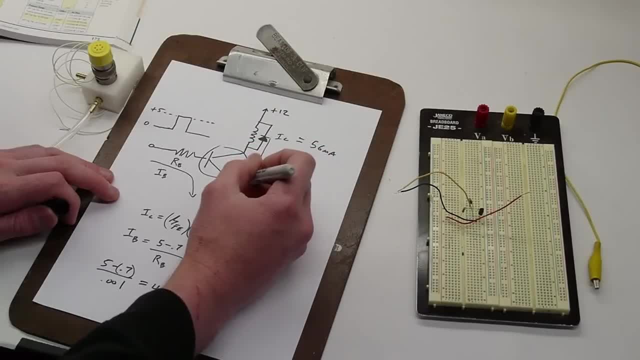 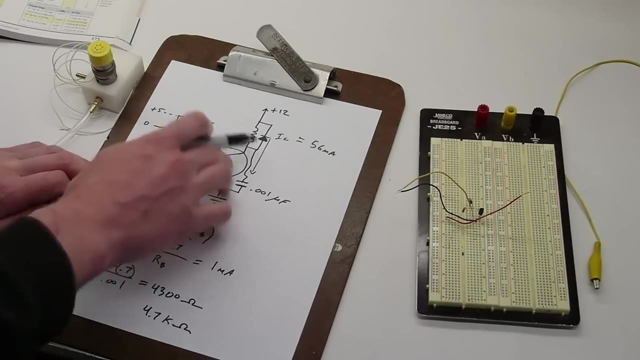 And you can also take it one step further and add a capacitor in there as well, like this, And this can be small like .001.. And the capacitor will smooth out the pulse here and give the diode time to turn on and make sure that there's absolutely no spiking or voltage rising going on in here. 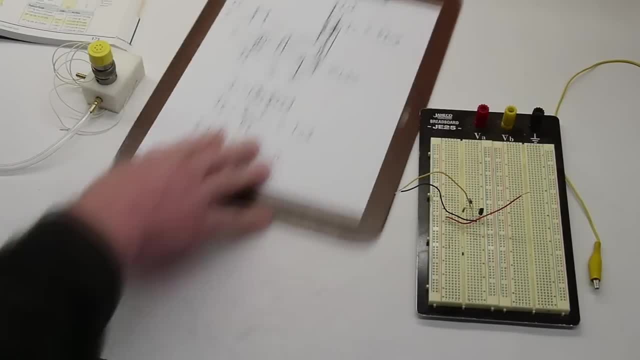 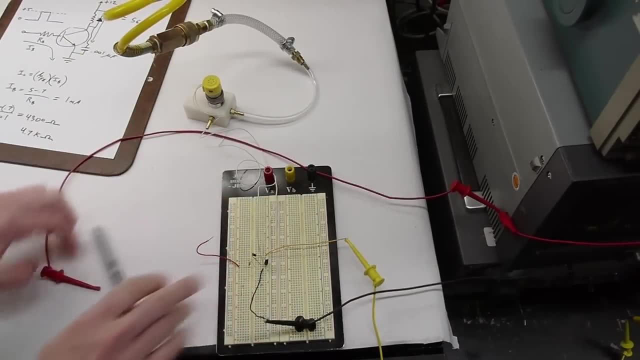 So let's build it and test it and prove that the thing actually works. Okay, so here's the circuit. Yellow is plus 12 volts, Black is a common ground And red is plus 5.. We've got our transistor here, the PN2222A. 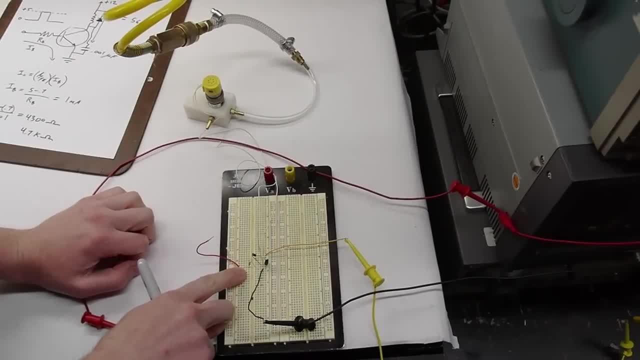 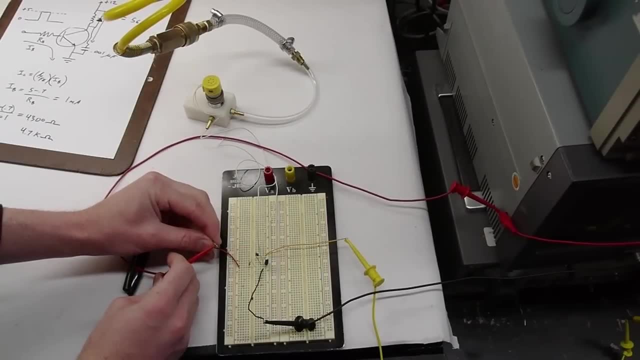 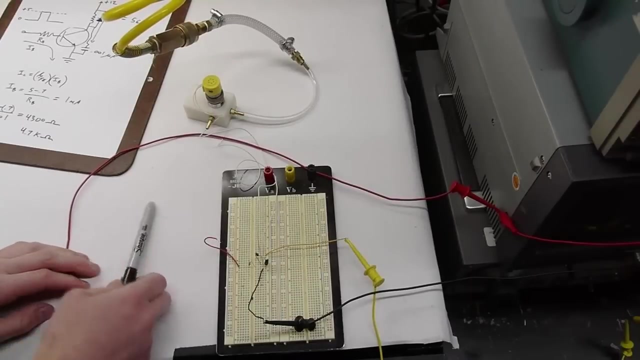 4.5 volts. 4.5 volts, 4.7K base resistor And our clamp diode. So if we put 5 volts into the resistor, control the valve quite nicely. So what we've done here is, taken a very, very small signal, 5 volts at 1 milliamp or less. 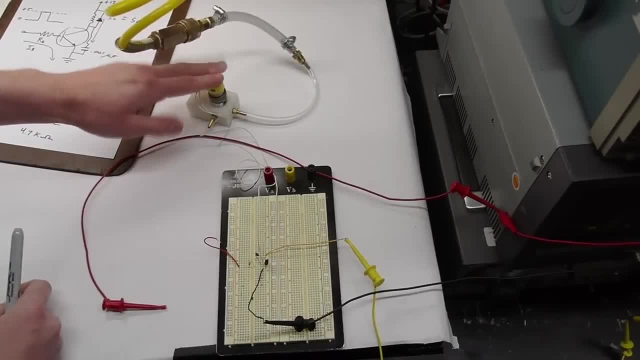 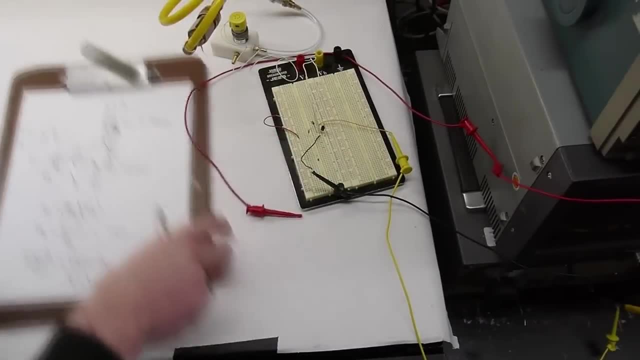 and are able to control. admittedly a pretty small signal, but we've taken care of the inductive kick from the solenoid valve. So I thought of just a couple of other things you might be wondering about. Throughout this. I was kind of trying to get the base resistor value chosen, and you might 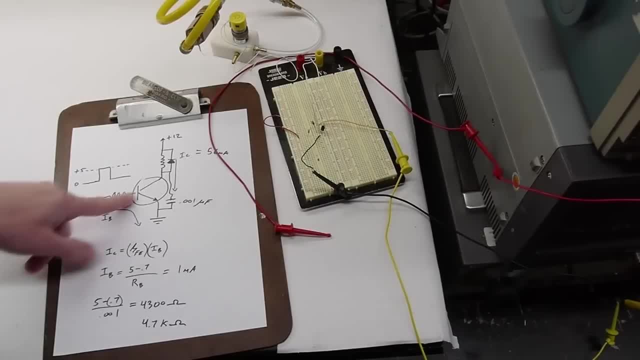 be thinking: well, screw it, We'll just put a zero ohm resistor, We'll just short this thing out and make sure we have enough base current. But unfortunately you can't do that because the transistor will draw so much current through the base it will destroy itself. 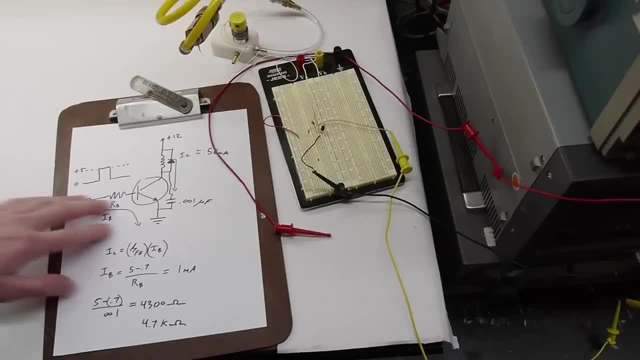 So. so you have to have a resistor here, or else the transistor will self-destruct. the very first time you test it you use it. in fact, when I was getting started in electronics, you know I thought a transistor was basically just a voltage controlled device, and so yeah. 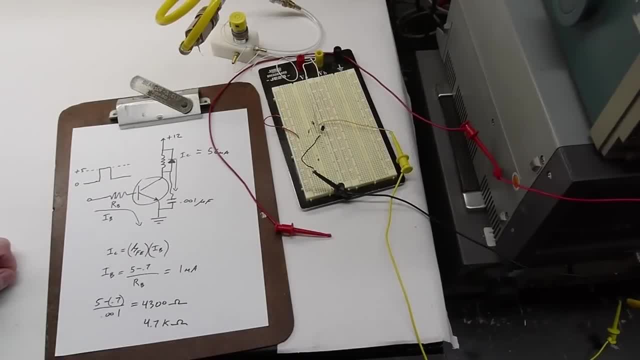 I put five volts on that base and, oddly enough, it didn't do anything. it didn't switch, didn't allow current to flow. so I tried another one, the same thing, and I thought, man, these transistors are just totally defective. but as it turns out, they were just being destroyed instantly. so, yeah, you have to have a base resistor. 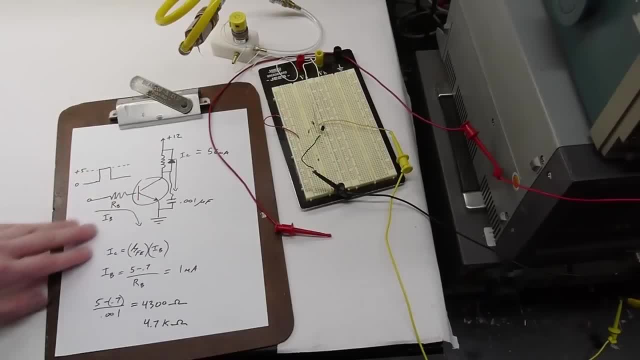 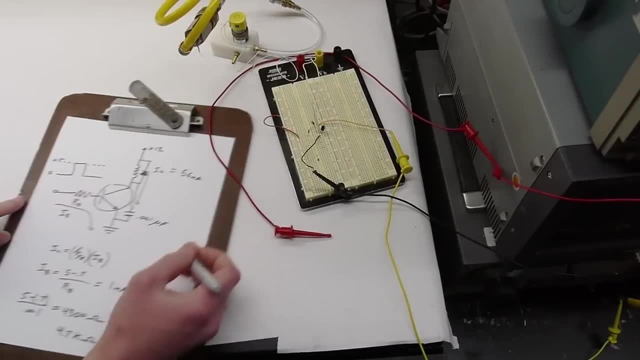 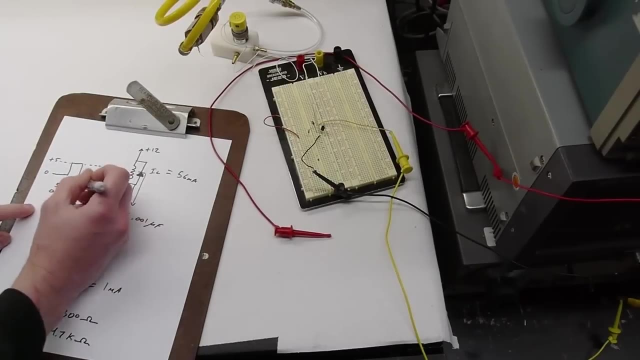 here. also there's going to be a voltage drop across here. so so I said that there's a point seven voltage drop here. so if we measure all these voltages, we've got five volts here, we got zero volts here, we've got point seven volts here. that's, you know, five minus point seven over RB, across. this resistor gives. 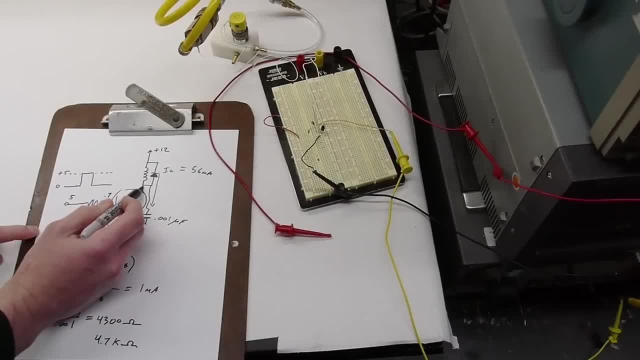 the current flow through here. but what's the voltage right here? this is actually pretty interesting. this. this voltage could be close to zero, or it could be about point one or point two volts, depending on the transistor and how much current is flowing through it. so I said that the reason we have a point seven volt drop. 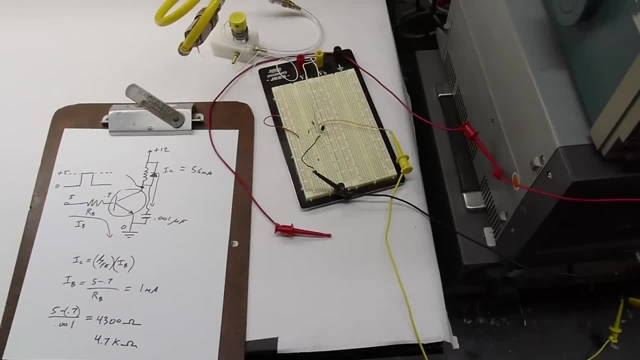 from the base to the emitter is because that's the way silicon semi conductors are built. we've got a pn-junction here. throughout the from from the collector to emitter there's a PN and an NP junction, so that point seven volts cancels itself out. so